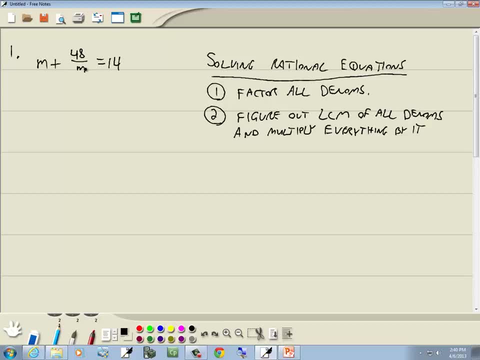 The greatest number of single M's in any denominator? Well, the greatest number. there's one here. so the greatest number of M's in any single denominator is one. So we're going to multiply everything by M. Now, when I say everything, I'm talking about what's separated by pluses and minuses and equals. 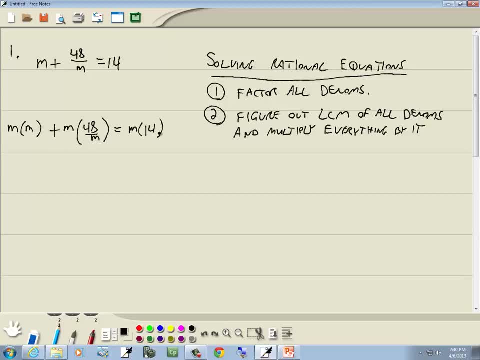 So we're going to multiply the M by M, the 48 over M by M and the 14 by M. Now this M cancels with this M M times M is M squared plus 48 equals 14M, And three says solve, and usually I put solve for X, but we'll just say solve. 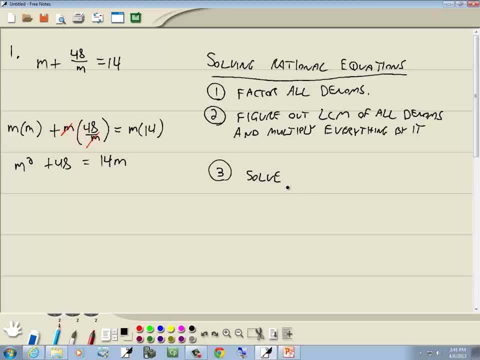 And that's pretty vague. That's what we're doing initially. We're solving, But every problem will be different. This one has an M squared, so it has a quadratic. But when you have a quadratic, you want to get everything over one side, zero on the other, and see if you can factor it. 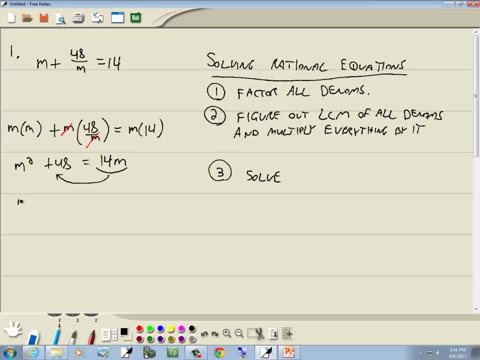 So I take the 14M over and we get M squared minus 14M plus 48 equals zero. Now, to factor this, we're going to use the PSD because we've got M squared, M, no M and there's no number in front of the M squared. 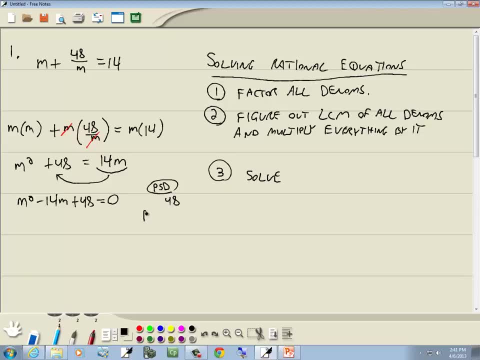 With PSD, we take the number at the end of 48 and we ignore signs. So if there's a negative 48, we'll still just take 48. And we come up with our three columns, Our P column, S column and D column. 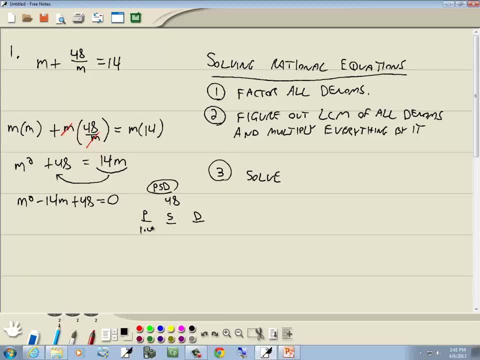 P. we list all. the product gives us 48. We've got 1 times 48,, 2 times 24,, 3 times 16,, 4 times 12,, 6 times 8.. In the S column we add these together. 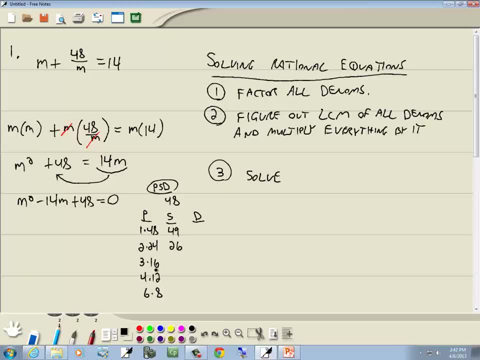 1 plus 48 is 49,. 2 plus 24 is 26,. 3 plus 16 is 19,. 4 plus 12 is 16.. 6 plus 8 is 14.. Difference column: we subtract smaller from larger. 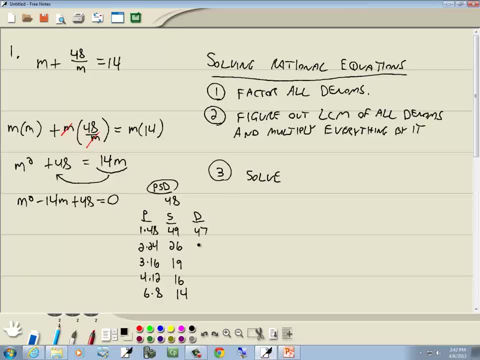 48 minus 1 is 47.. 24 minus 2 is 22.. 16 minus 3 is 13.. 12 minus 4 is 8.. And 8 minus 6 is 2.. The number we're looking for is the number in our middle term, which is 14.. 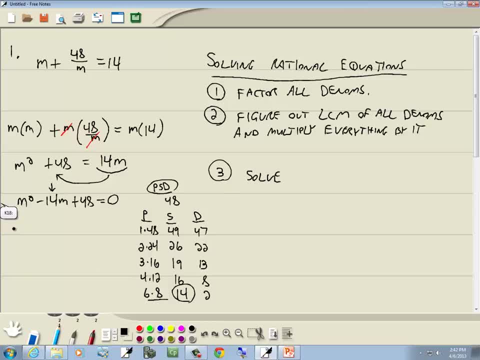 Which is right here. So we're going to use 6 and 8.. Now our larger number in the P column that we're using is 14.. So we're going to use 6 and 8.. Now our larger number in the P column that we're using is 16.. 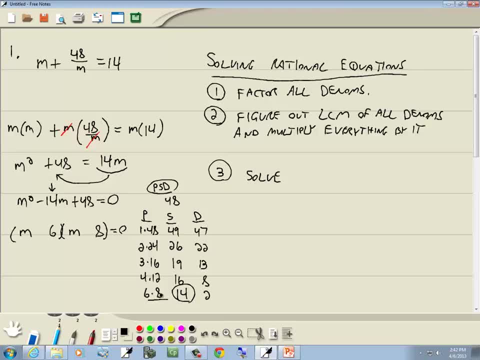 Now our larger number in the P column that we're using is 16.. So we're going to use 6, and P, Which we're using, which is the 8, will always be the same sign as the middle term, which is negative. 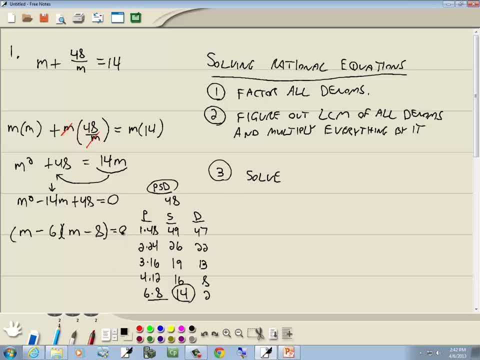 The number alsoittä circled in the S column, S, for same signs. So if the 8 is negative, the 6 is negative. Now, zero factor property. So you get zero on one side. you factor to the other side. you set each factor equal to 0.. 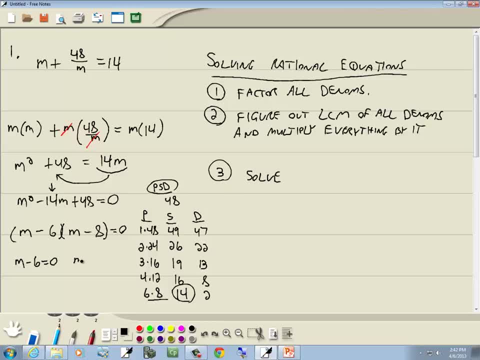 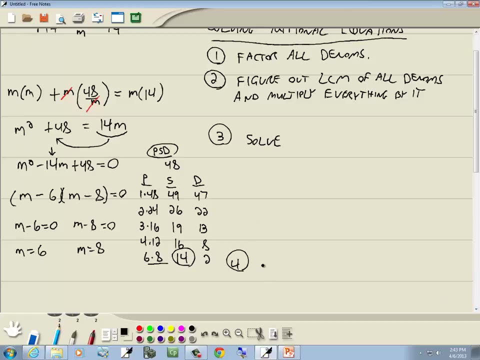 So I'll set M minus 6 equal to 0, and M minus 8 equal to 0. And we solve those and we get M is equal to 6 and M is equal to 8.. now step four: semi check your answer. so semi check your answers now. what I mean by that is: 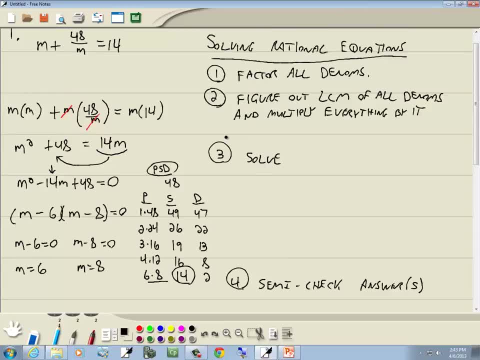 you don't need to let fully check it, but you want to make sure that when you plug those values back in they don't cause a denominator equals zero. for example, if I put six in for the M, put six here, put six here, forty eight over six, well, that doesn't cause a zero in denominator. so 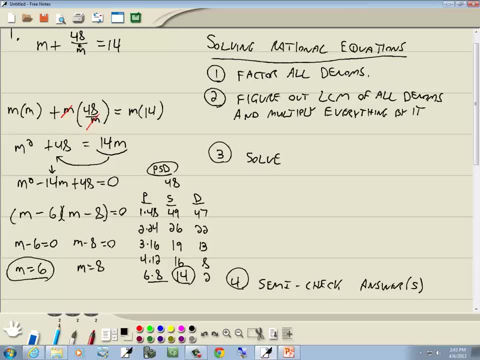 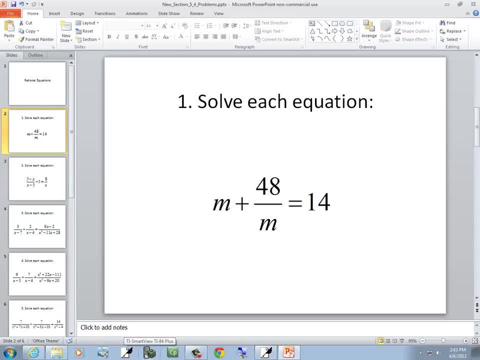 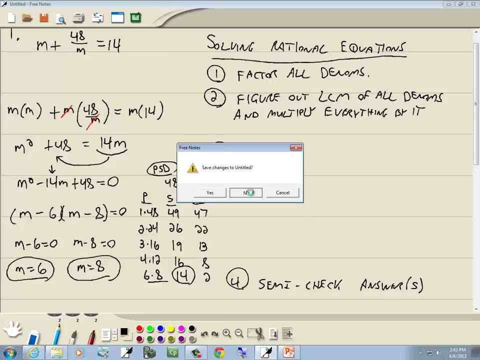 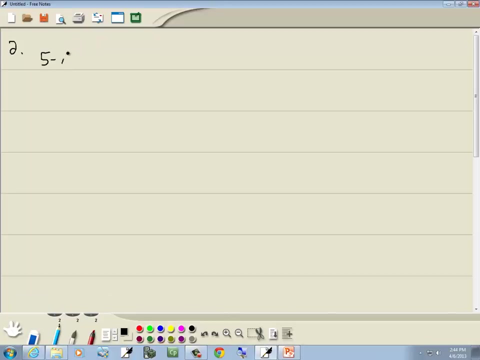 that's the answer. if we put eight in here, forty eight over eight, well that our denominator still not zero, so both of those actually work. let's take a look at our next problem. five minus X over X. minus five plus five equals eight over X. this one's actually got a shortcut that I'm going. 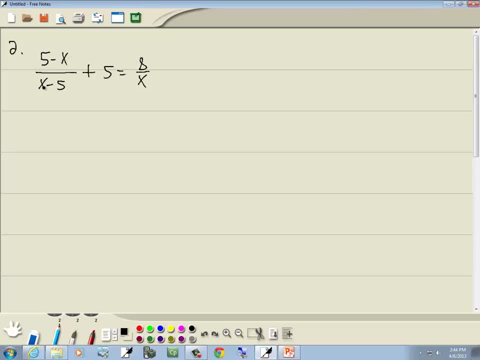 to ignore. notice how this is five minus X and this is X minus five. well, if I were to factor out a negative one up on top, what I'd find is that all this fraction here gives us negative one. so we'd have negative one plus five, which gives us four. I'd like steps to work 100% of time or as close. 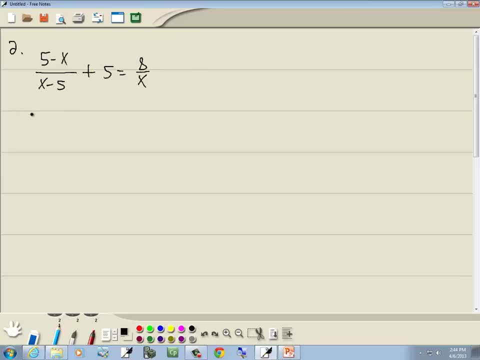 as possible, though, so I'm going to ignore short shortcuts. okay, first step: factor all your denominators. now we got X minus five and X. there's nothing to factor. step two: figure out our LCM. realize that the single X here is different than this X over here. 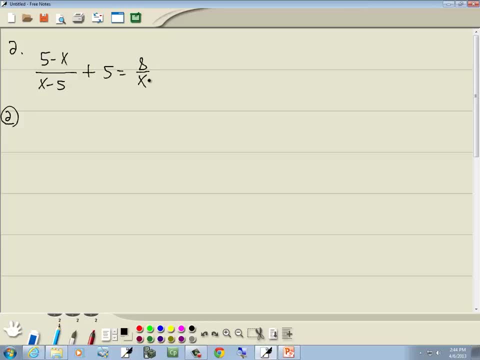 so we'll start with our first factor. we'll start with X, and I'm looking for the greatest number of single X's in any single denominator. there's none here, there's one here, so we'll have one X. I go to my next factor, the X minus five. 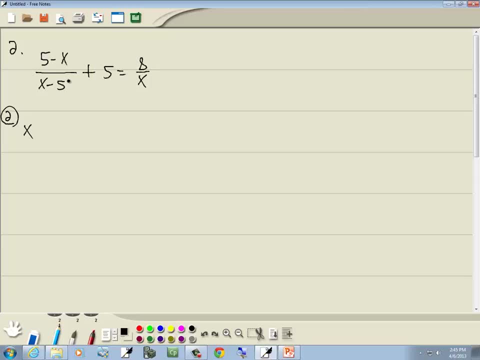 now I'm looking for the greatest number of X minus fives in a single denominator. there's one here, none here, so we'll use one. the answer to that will almost always be one when I ask you: how many of these do you have in a single denominator? so that's our LCM and that's what we'll part thing by. 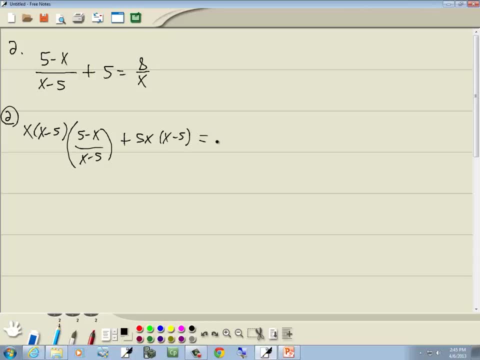 and again, when I say everything, I'm talking about what's separated by pluses and minuses. okay, well, this X minus five here cancels this X minus five. this X here cancels of this X, and so we're left with. I'll write it down, then I'll multiply it through: we're left with X times. 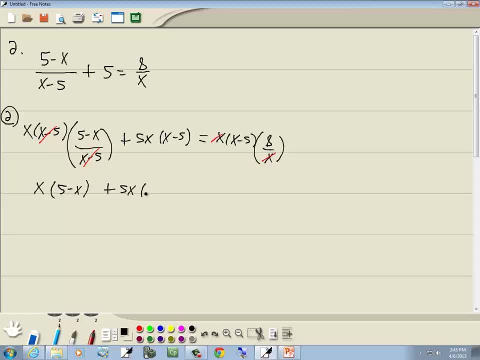 five minus X plus five X times X minus five equals eight times X minus five. well, X times five is 5X X times negative. X is negative. X squared plus 5X times X is 5X squared 5X times negative. five gives us negative 25X. 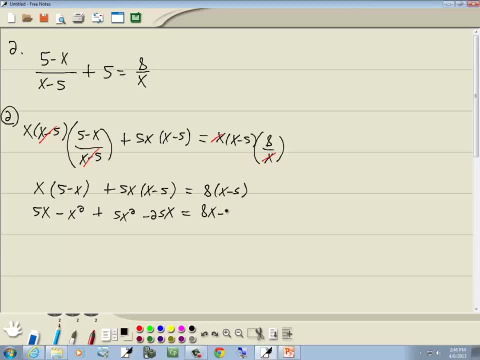 equals eight times X is 8X. 8 times negative. 5 is negative 40.. now we want to combine together like terms at a step. here we have a negative X squared plus 5X squared. that gives us 4X squared. 5X minus 25X gives us negative 20X equals 8X minus 40.. 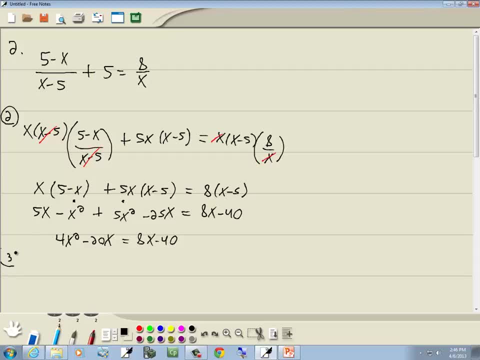 now step three is we want to solve- in this case we want to solve for X, and we have a quadratic, we have an X squared, so we won't get everything over one side, zero on the other. so I'll take the 8X minus 40 over. so we've got 4X squared minus 20X, minus 8X plus 40, equal to zero. 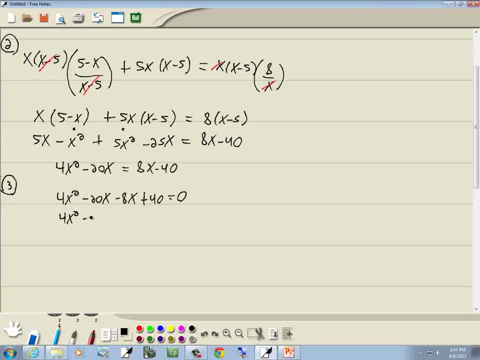 which gives us 4X squared minus 28X plus 40, equal to zero. well, the first thing I can do is I can factor out a GCF. they're all divisible by four, so I'll bring a four out, and that leaves us X squared minus 7X plus 10, equals zero. now, 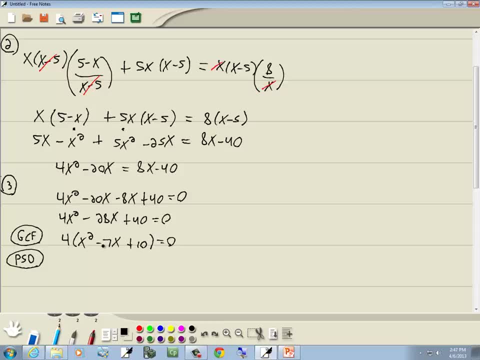 what's inside the parentheses is going to be PSD, because we have X squared, X, no X. there's no number in front of the X squared. so I'll take the 10, come over here and I'll create my three columns: my P column, my S column and D column. and the P column will list all products. give us 10. we. 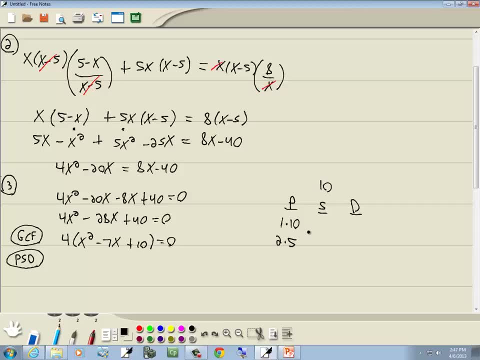 got 1 times 10, 2 times 5 and the S column. we add those together: 1 plus 10 is 11, 2 plus 5 is 7 and the difference column will subtract them. 10 minus 1 is 9, 5 minus 2 is 3.. now the number we're looking. 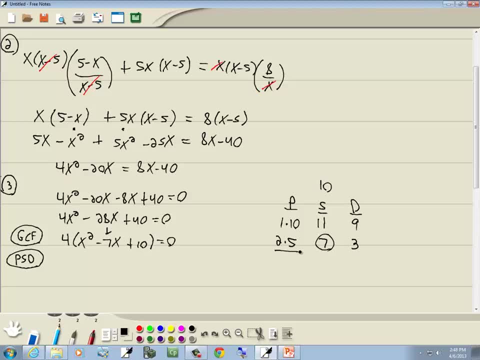 for is a number in our middle term, which is a 7, which is right here. so we're going to use 2 and 5. the 4 carries down, it doesn't change anything, but we have to keep carrying it down and we use 2 and 5.. now our larger number in the P column, that 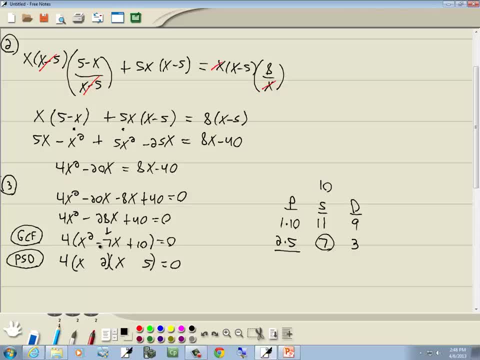 we're using, which is 5, will always be the same size of middle term, which was negative the number I circled in the S column S for same sign. so if the five is negative, the two will be negative. now the zero factor property says you get zero on one side, you factor the other side. 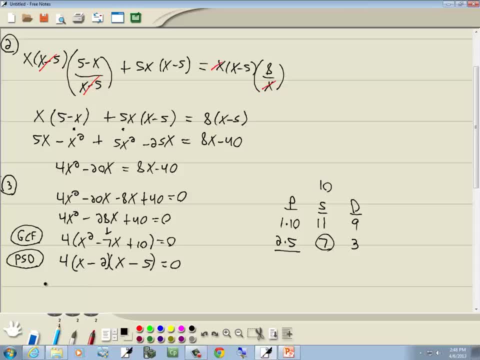 you set each factor equal to zero. now it never does this any good to set the number equal to zero. so if I set four equal to zero, there's no X to solve for, so that goes nowhere. so we'll set X minus two equals zero and X minus five equal to zero, and we get X is equal to two and X is equal to five. 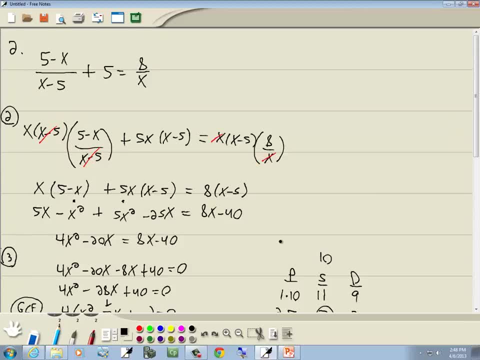 well, step four: semi-check your answers. if I take the two, put it up in my original problem, two minus five, that's not zero. but put two here, it's not zero, so that one's fine. now if I take the X equals five and plug it back up here, if I put five in for X, I get five minus five. 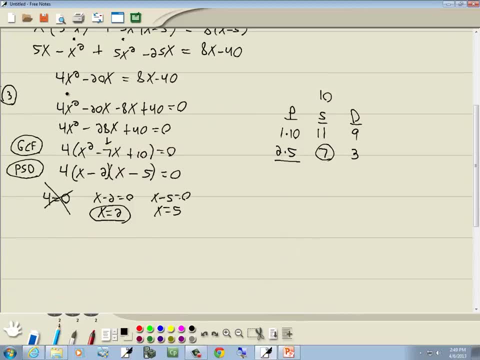 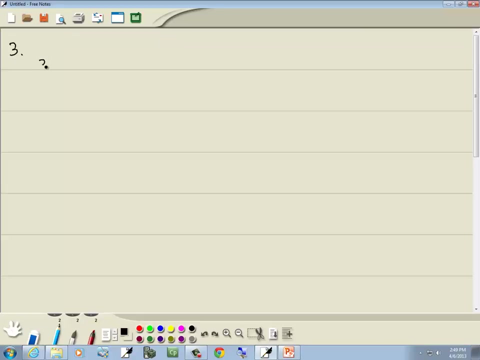 in the first fraction here, which gives a zero. so this one causes a zero in denominator, so we're going to cross that one out. so our only answer is: X equals two. let's take a look at this: one, the, the three, three over X minus seven, plus two over X minus four. 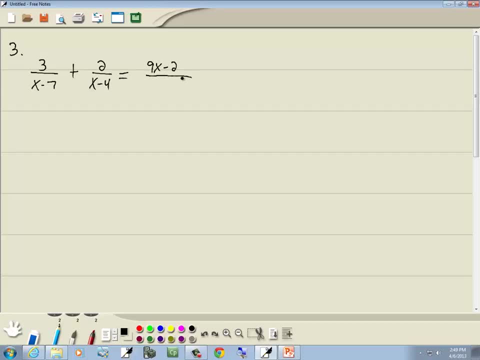 equals nine X minus two over X squared minus 11, X plus 28.. step one: uh, factor all of our denominators: X minus seven, we can't do anything with. X minus four, we can't do anything with. but the X squared minus 11, X plus 28 is the PST method. 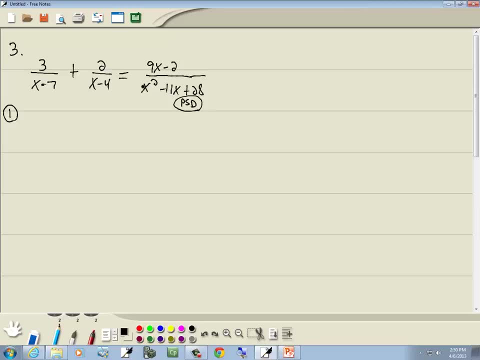 because it's X squared X, no, X, no number in front of the X squared PST. we'll take the number at the end, 28, and we'll come up with our three columns. P column: we write: all products give us 28. we got 1 times 28, 2 times 14, 3, no, 4 times 7.. in the S column we add them together: 1 plus 28 is 29, 2 plus. 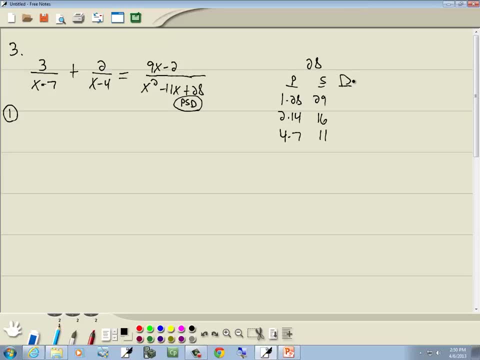 14 is 16. 4 plus 7 is 11.. difference column will subtract them smaller from larger: 28 minus 1 is 27.. one plus 28 is 29. two plus 14 is 16. 4 plus 7 is 11. difference column will subtract them smaller from larger: 28 minus 1. 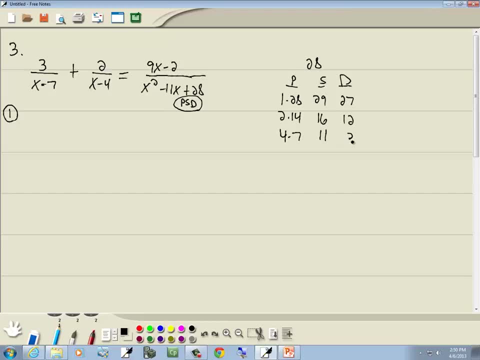 27.. 14 minus 2 is 12.. 7 minus 4 is 3.. Now the number we're looking for is the number on our middle term, which is 11,, which is right there. so we'll use 4 and 7.. 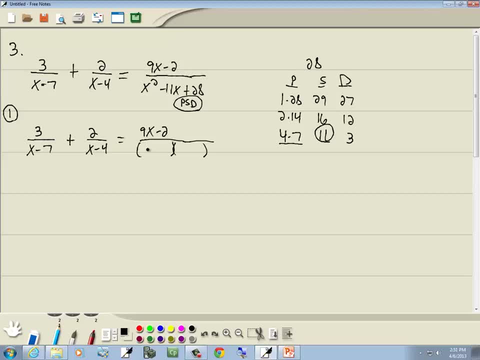 So this factors: This is x, this is x. We're using 4 and 7, so put 4 and 7 in there. Now, our larger number in the p column that we're using, which is the 7, will always be the same sign as the middle term. Well, middle term is negative: 11x. 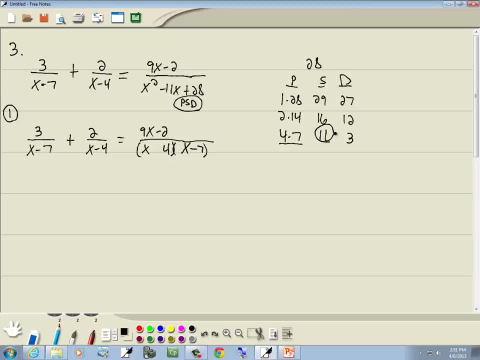 so it's negative. The number I circled is in the s column s for same sign. so if the 7 is negative, the 4 has to be negative. Step 2. Figure out your LCM and multiply everything by it. Let's start with our first factor, the x minus. 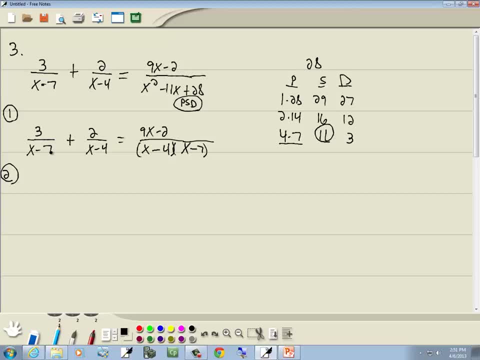 7.. Now we're looking for the greatest number of x minus 7s in any single denominator. There's 1 here, None here, 1 here. So the greatest number of x minus 7s in any single denominator is 1.. 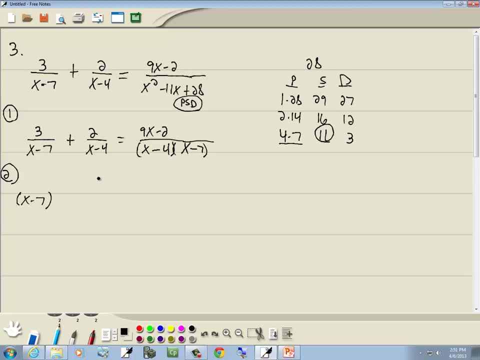 Then we'll go to our next factor, the x minus 4.. Now I'm looking for the greatest number of x minus 4s in any single denominator. There's none here. 1 here, 1 here. So the greatest number of x minus 4s in any single denominator. 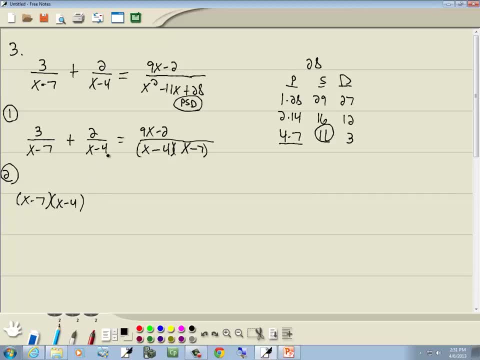 is 1.. Again, the answer to that question will almost always be 1.. So we'll multiply that times our first fraction, And we'll multiply it times our second fraction, And we'll multiply it times our fraction on the right side. 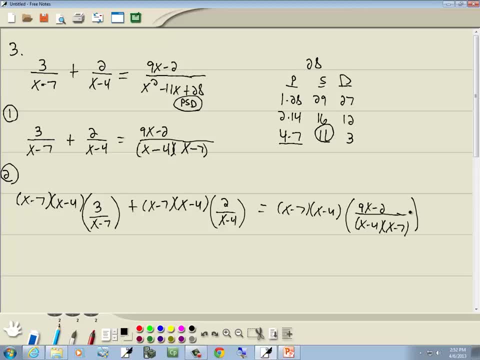 Okay, Taking my glasses off Kind of bothered me, Gave me a headache, Let's cancel. So this x minus 7 cancels that x minus 7.. This x minus 4 cancels that x minus 4.. This x minus 7 cancels that x minus 7.. This x minus 4 cancels that x minus 4.. 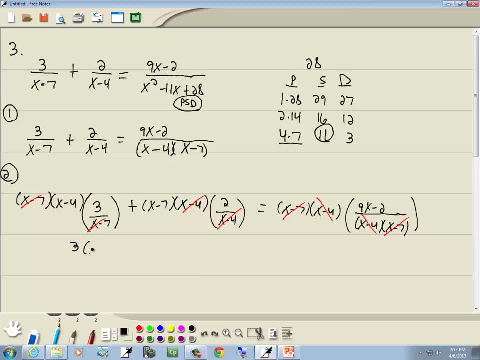 Let me write down what I have left and then I'll take it from there. So I've got: 3 times x minus 4, plus 2 times x minus 7 equals 9x minus 2.. Well, 3 times x is 3x. 3 times negative 4 is negative 12.. 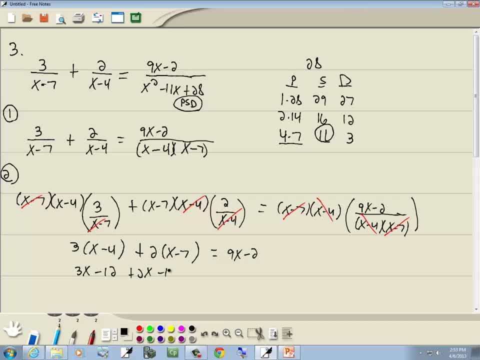 2 times x is 2x And 2 times negative 7 is negative 14.. That equals 9x minus 2.. And again, no matter where you are in math, you show it's combined together like terms, numbers. 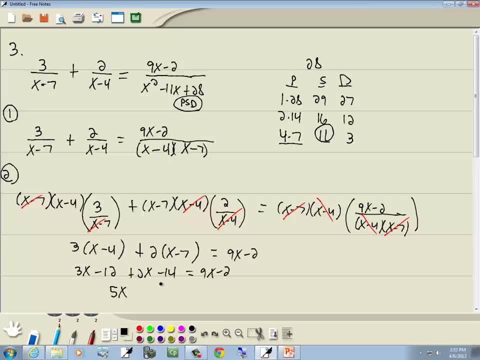 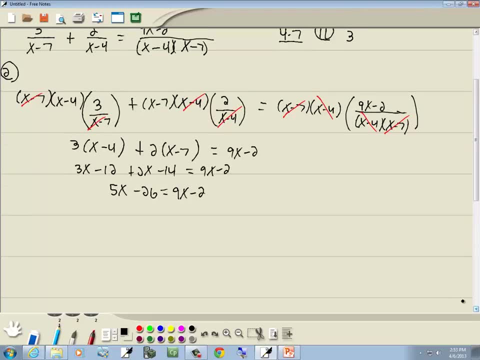 3x plus 2x is 5x. Negative 12 and negative 14 gives me negative 26.. Okay, Step 3.. We want to solve for x. This time. this is a linear equation. Linear equation because everything is the first power. 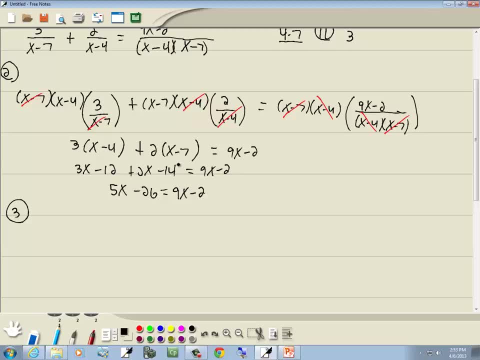 x is the first. We don't have an x squared. Well, linear equations, you know: first step, give your parentheses. Second step: give your fractions. Third step: give everything with an x on one side. So I'll take the 9x over the left side. 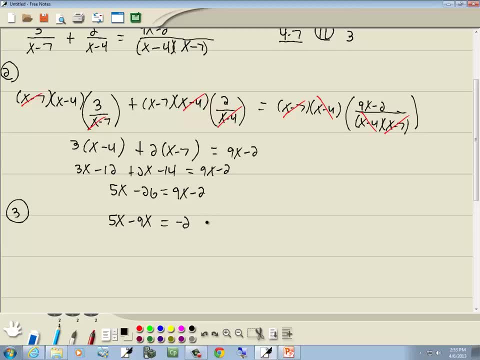 It becomes a negative 9x. I'll take the negative 26 to the right side: It becomes a positive 26.. Combine together like terms: 5x minus 9x is negative. 4x Negative. 2 plus 26 is 24.. 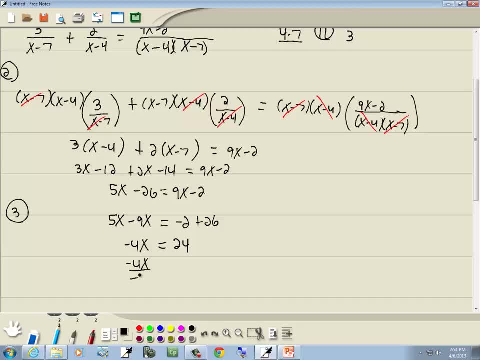 And last step is: divide both sides by negative 4.. And 24 divided by negative 4 gives us negative 6.. Maybe We need to semi-check our answers. And the x equals negative 6.. You can actually plug that in at step 1. 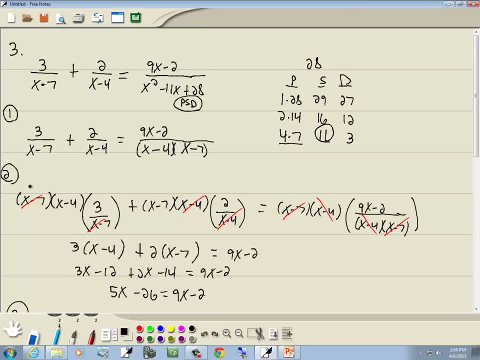 where you have everything factored. So if I put negative 6 in for the x here, I get negative 6 minus 7.. That's not 0.. Negative 6 minus 4.. That's not 0.. Negative 6 minus 4.. 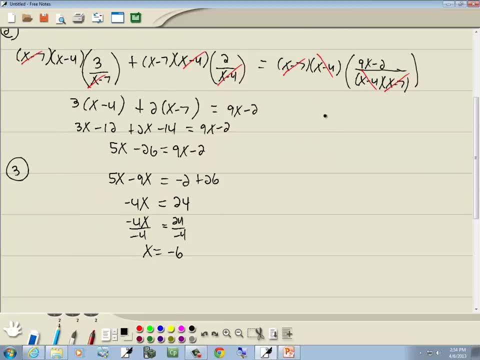 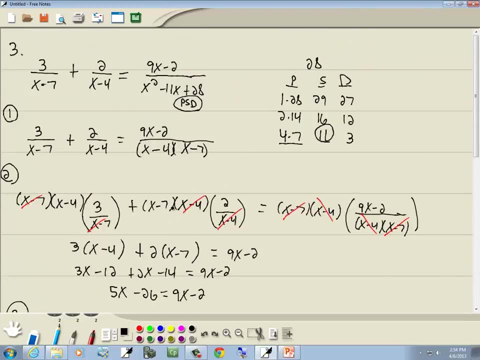 That's not 0. So I put negative 6 here and then put negative 7 up there. If this one actually checks, that's our answer. The values of what causes problems here is if we come up with: x equals 4,. 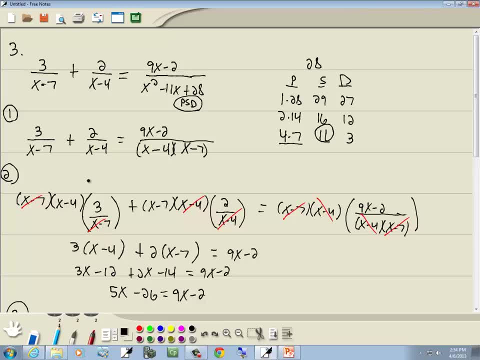 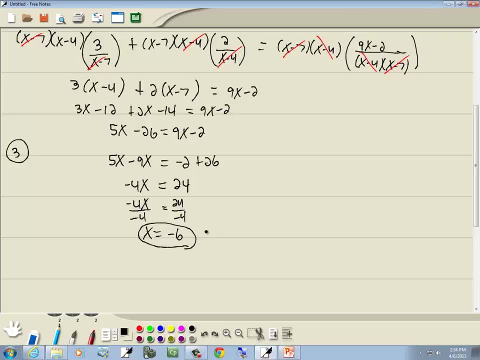 if I put 4 back up here, 4 minus 4 would give us 0.. Or if I come up with: x equals 7, 7 minus 7 gives us 0. So again, you need to semi-check it to see if your problem here is a –. 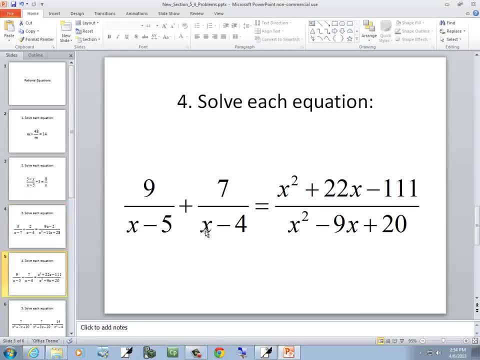 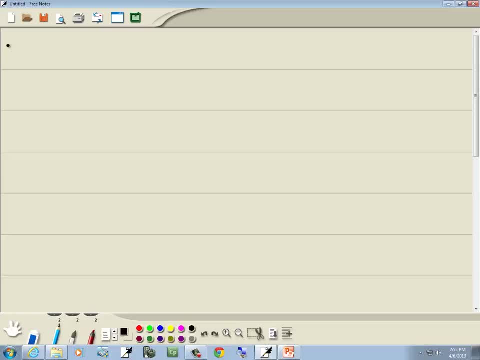 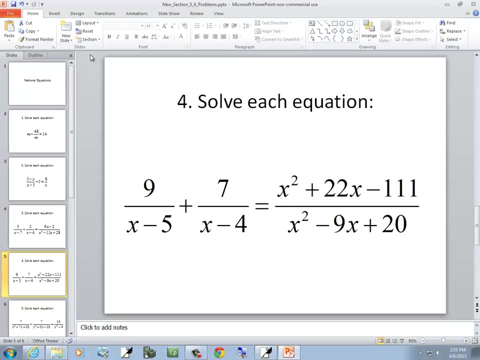 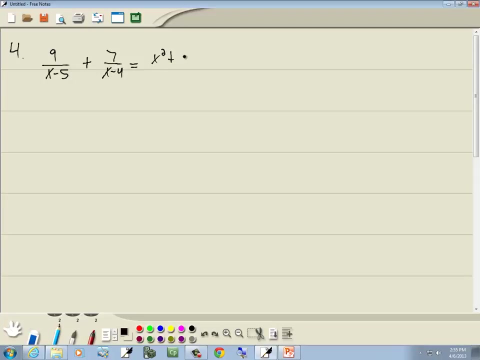 causes the denominator to equal 0.. Let's take a look at this one Problem, number four: nine over x minus five plus seven over x minus four equals x squared plus 22x minus 111 over x squared minus 9x plus 20.. 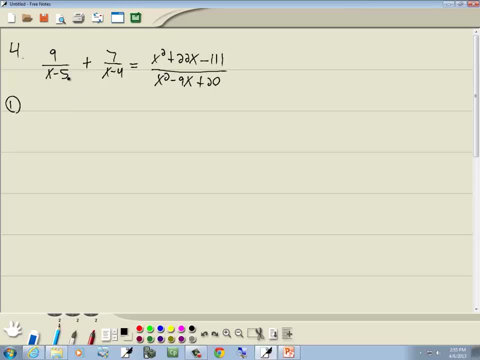 Step one: factor all our denominators, The x minus five, the x minus four I can't do anything with. But x squared minus 9x plus 20 is a PSD method, Because it's x squared x, no, x, no number in front of the x squared. 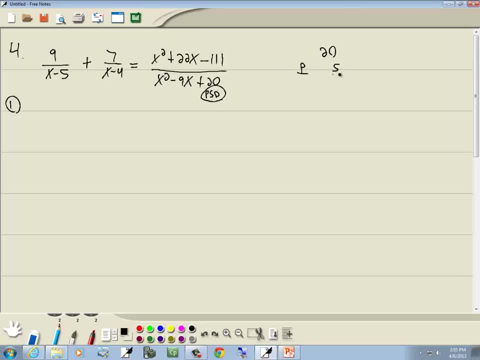 PSD. we take the number at the end, which is the 20, and we come up with our three columns. P column we list all products, give us 20.. We've got one times 20,, two times 10,, four times five. 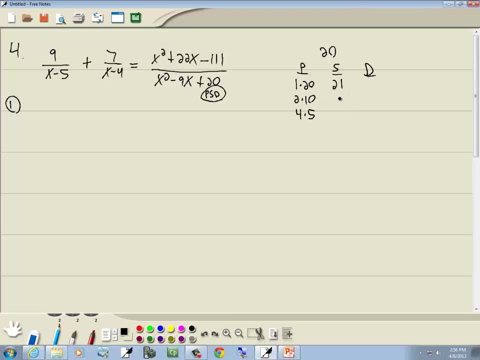 The S column. we add them together: One plus 20 is 21.. Two plus 10 is 12.. Four plus five is nine. Difference column. we subtract them smaller from larger: 20 minus one is 19.. 10 minus two is eight. 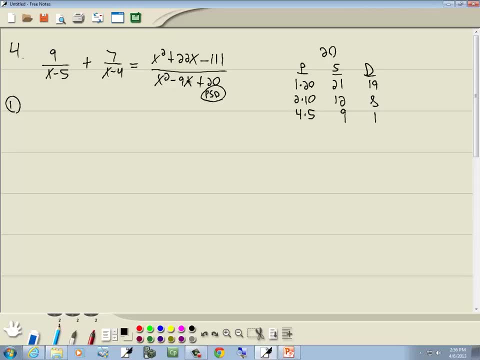 Five minus four is one. The number we're looking for is the number in our middle term, which is nine, which is right here. So we're going to use four and five. Everything else remains exactly as is. Now. we're going to use four and five. 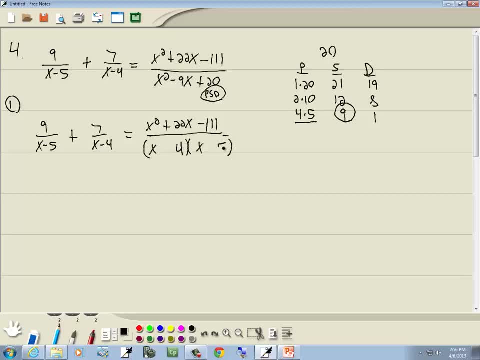 So that's x, that's x. we're going to use four and five. Now, our larger number that we're using in the P column, which is five, is always going to be the same sign as the middle term, which is negative: 9x. so it's negative. 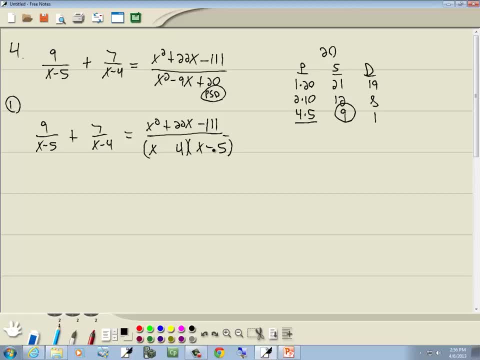 The number. I circled in the S column S for same sign. so if the five is negative, the four is negative. Step two: figure out your LCM. Let's do that first. We'll start with our first factor, the exponent. 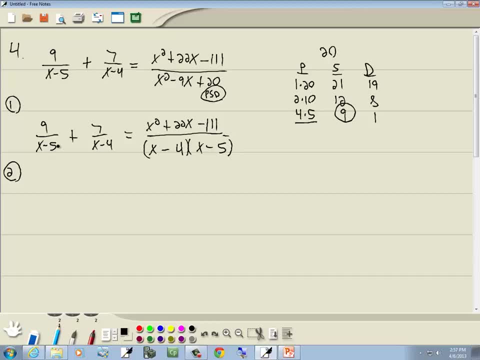 x minus five, And we're looking for the greatest number of x minus five, as in any single denominator. There's one here, none here, one here. So the greatest number of x minus five, as in any single denominator, is one. Then we'll go to our next one, the x minus four. 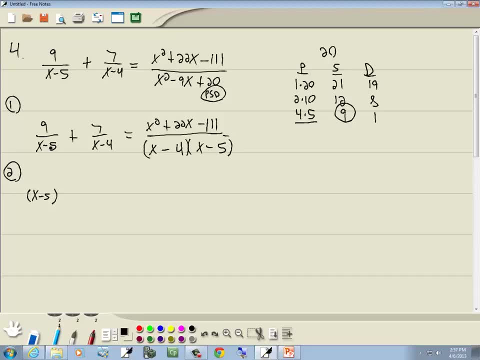 We're looking for the greatest number of x minus four, as in any single denominator. There's none here, there's one here, there's one here. So the greatest number of x minus four, as in any single denominator, is one. So our LCM is x minus five, x minus four. 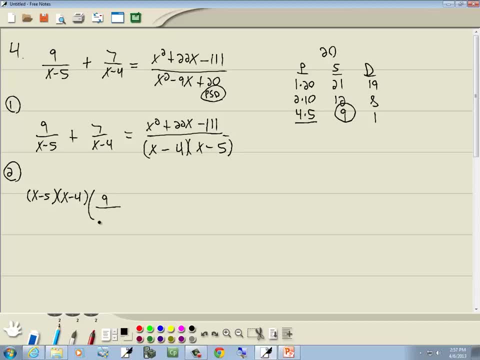 And that's what we'll multiply everything by. So we'll multiply it by nine over x minus five. We'll multiply it times seven over x minus four. And we'll multiply it times x squared plus 22x minus 111 over x minus four. x minus five. 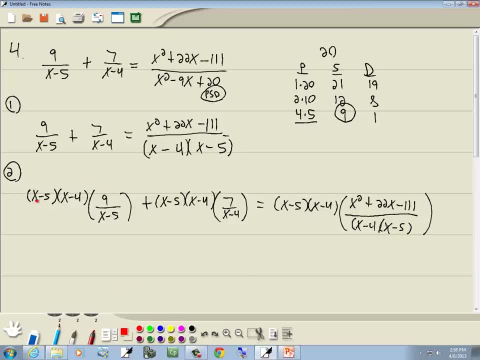 Well, let's see what cancels The x minus five there. cancels that x minus five, This x minus four. cancels that x minus four, This x minus five, this x minus five, this x minus four, this x minus four. 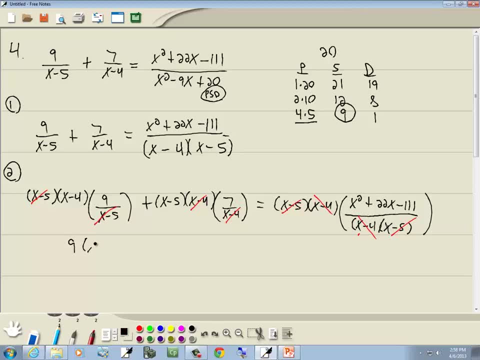 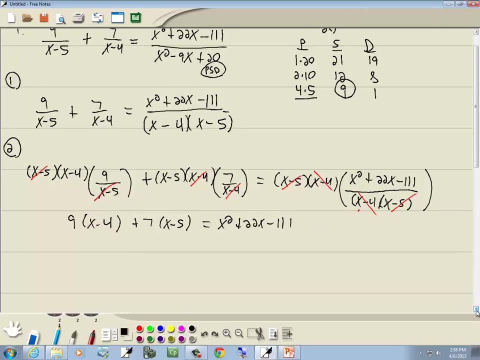 So let's write down what we have left before we multiply through. So we've got nine times x minus four, plus seven times x minus five equals x squared plus 22x Minus 111.. Well, nine times x is 9x. 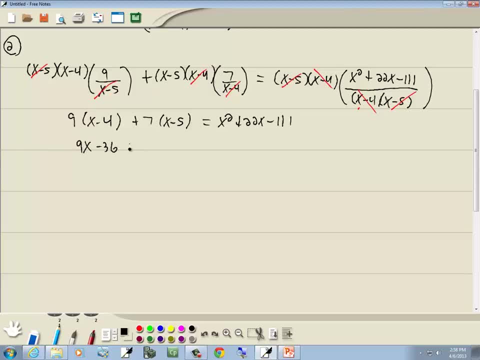 Nine times negative. four is negative 36.. Seven times x is 7x. Seven times negative five is negative 35.. Equals x squared plus 22x minus 111.. Combine together like terms: 9x plus 7x is 16x. 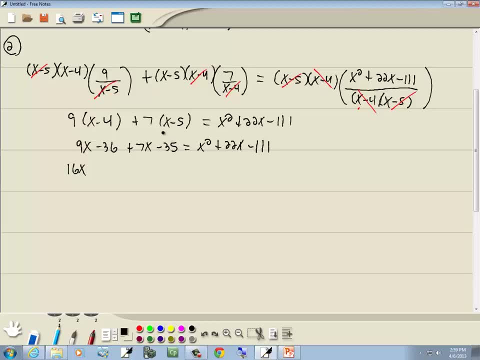 Negative 36, negative 35 is negative 71.. Equals: x squared plus 22x minus 111.. Now step three. solve for x. Well, this has an x squared in it, a quadratic. So we want to get everything over one side, zero on the other. 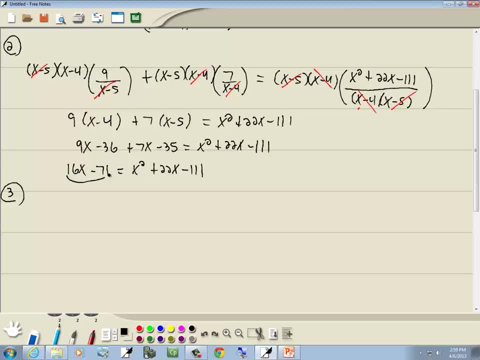 And we'd like the number that's in front of our x squared to be positive. So I'm going to take the 16x minus 71 over to the right side. So we've got. zero is equal to x squared plus 22x minus 16x. 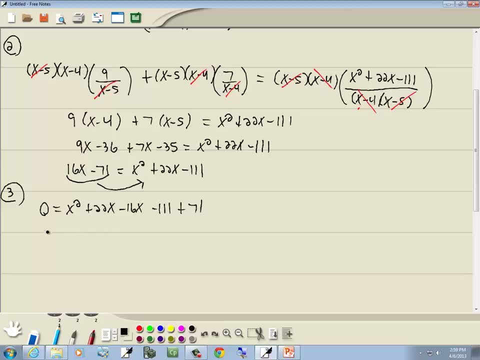 Minus 111 plus 71.. Again, you take anything across here equals your sign changes. Combine together like terms: 22x minus 16x is plus 6x. Negative. 111 plus 71 is negative 40.. Yeah, negative 40.. 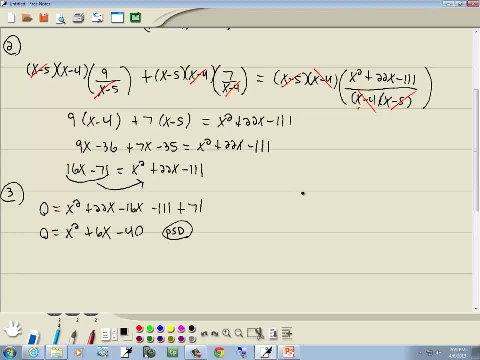 Well, now we can factor this using the PSD method. Take our number at the end, the 40., And come up with our three columns. Write down all products, give us 40. We've got 1 times 40.. 2 times 20.. 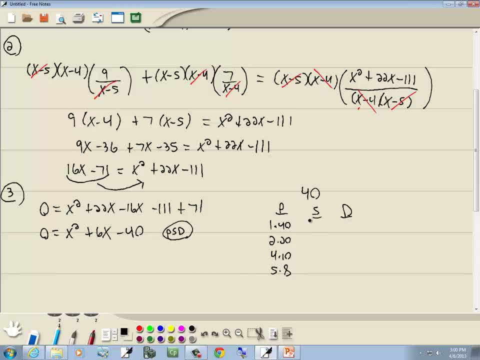 4 times 10.. 5 times 8.. We want to add these: 1 plus 40 is 41.. That's the S column. 2 plus 20 is 22.. 4 plus 10 is 14.. 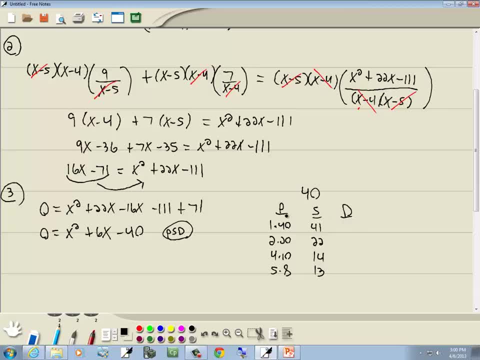 5 plus 8 is 13.. Difference column Subtract smaller from larger: 40 minus 1 is 39.. 20 minus 2 is 18.. 10 minus 4 is 6.. 8 minus 5 is 3.. 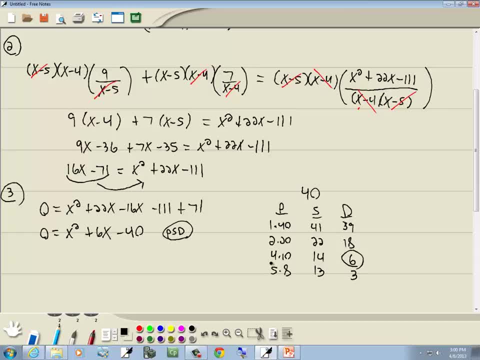 Now, the number we're looking for is the number in our middle term, which is 6.. So we're going to use 4 and 10.. Now our larger number in the P column that we're going to use, which is the 10,. 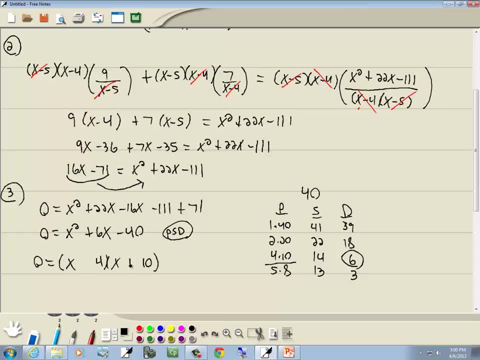 is always going to be the same sign as the middle term, which is positive. The number I circled is in the difference column D for different signs. So if the 10 is positive, then the 4 has to be negative. 0 factor property. 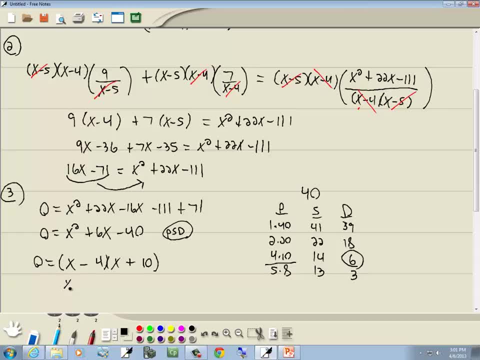 You get 0 on one side, You factor the other side, You set each factor equal to 0. So I'll set x minus 4 equal to 0 and x plus 10 equal to 0. And that gives us x equals 4 and x equals negative 10, maybe. 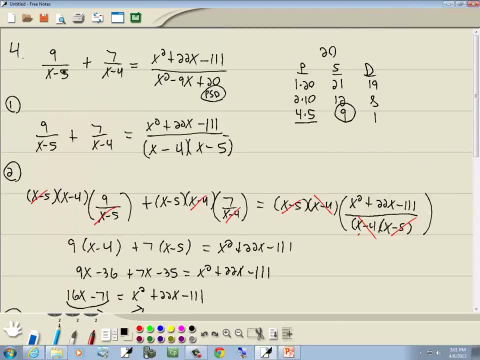 We want to check it, So I'm going to check the x equals 4.. Go back up here. 4 minus 5 is negative 1. That's OK. 4 minus 4 here gives us 0 in the denominator. 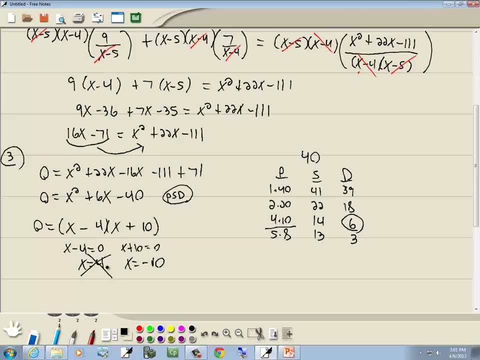 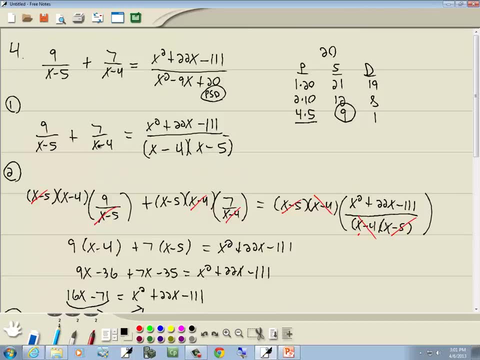 Can't have that. Negative 1 fails. Now if I take negative 10, put it back up here: Negative 10 minus 5, that's not 0.. Negative 10 minus 4, that's not 0.. And same thing over here. 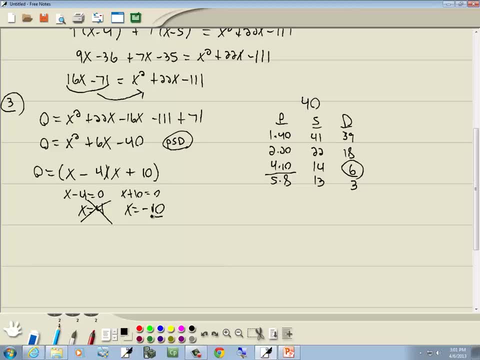 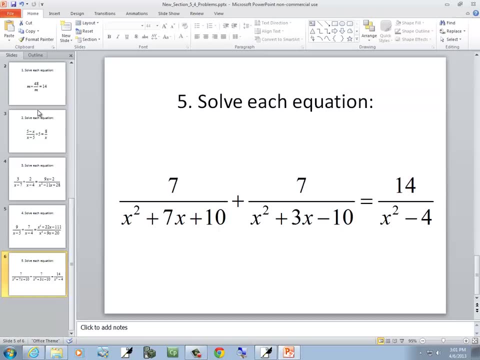 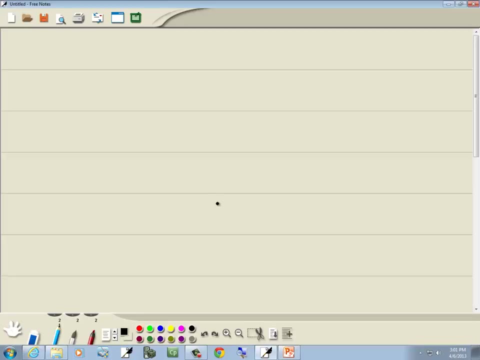 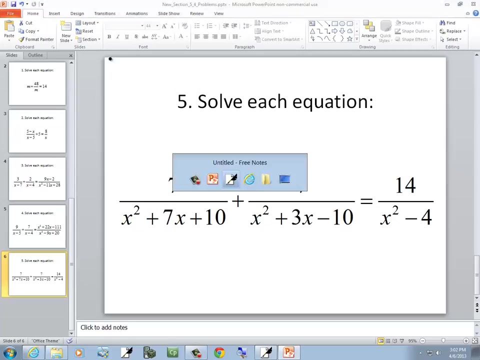 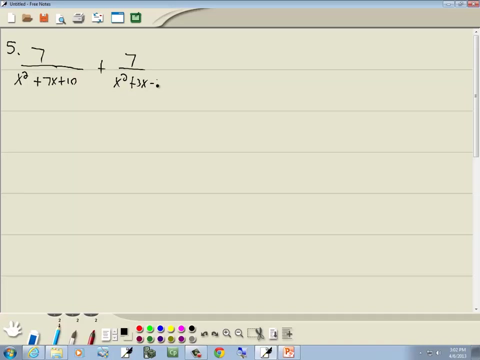 So that problem or that answer actually works. And let's look at our last problem. So I got 7 over x squared plus 7x plus 10 plus 7 over x squared plus 3x minus 10 equals 14 over x squared minus 10.. 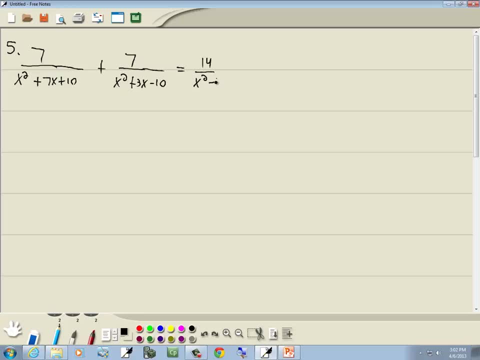 That's 0.. x squared minus 4.. Step 1. Factor all our denominators: This is a PSD because it's x squared, x, no x, no number in front of our x squared. This one is also a PSD. 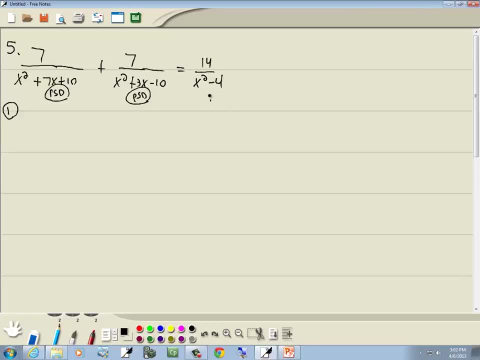 x squared, x, no, x. no number in front of our x squared. This one is dots Difference: two squares, Two terms of minus 3.. Well, both of these are 10, so that works out nice, PSD. we take our number at the end, ignoring signs, and come up with our three columns. 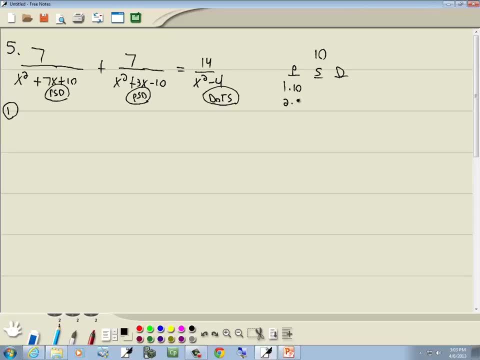 Write down all products, give us 10.. We've got 1 times 10, 2 times 5.. Add them: 1 plus 10 is 11.. 2 plus 5 is 7.. Subtract them: Difference column. 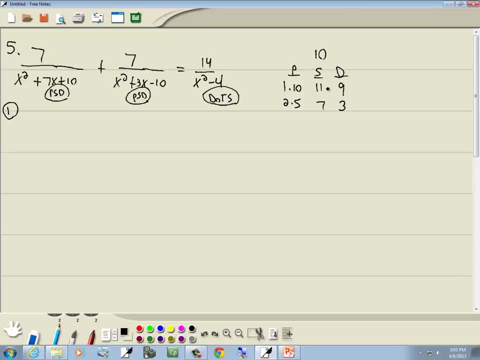 10 minus 1 is 9.. 5 minus 2 gives us 3.. Now, this first one we're looking for is 7. 7's right here. so we're going to use 2 and 5.. 2 and 5.. 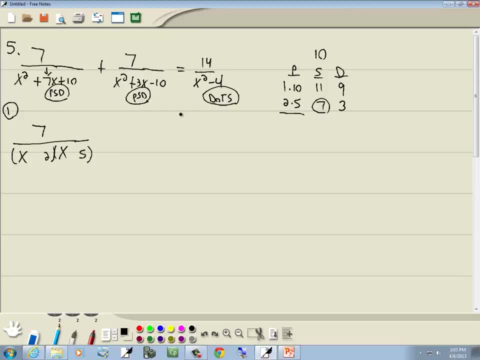 Now our larger number in the P column that we're using, which is the 5, is always going to be the same size as the middle term, which is positive Number. our circles in the S column S for same signs. so if this one's positive, the other one's positive. 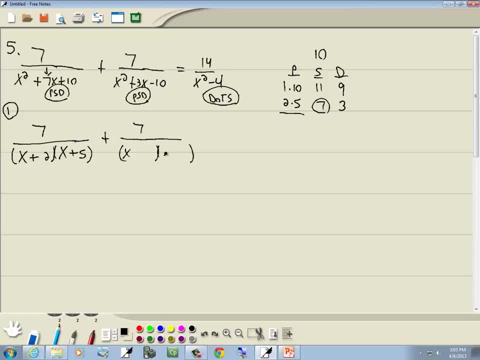 Now our second one. This one also uses 10.. The number in the middle is a 3, though, so we're looking for a 3.. Well, 3's. in this column We're going to use 2 and 5 again. 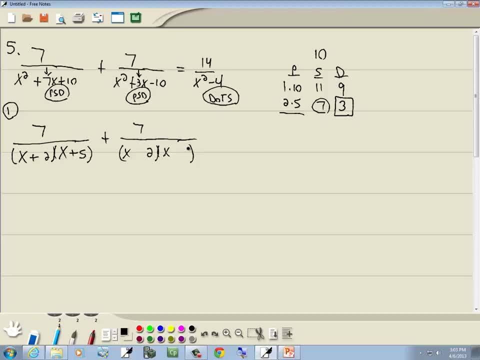 So we're going to use 2 and 5 again. Our larger number in the P column that we're using, which is the 5, is always going to be the same size as the middle term, which is positive. The number I put the box around is in the difference column D for different signs. so if the 5 is positive, then 2 is negative. 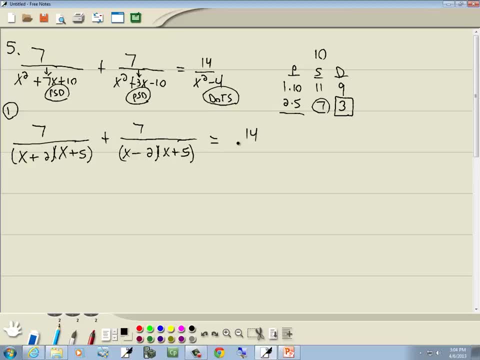 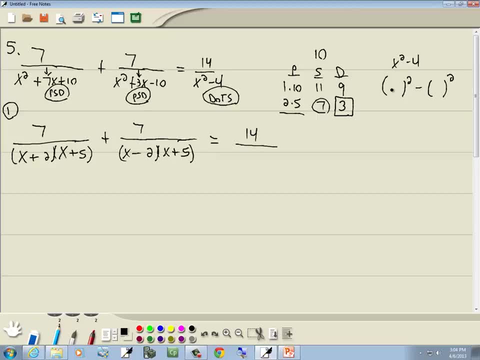 We'll start with the X squared. You ask yourself what times itself gives you the X squared, and that's X. And then we'll go to the 4, and you ask yourself what times itself gives you the 4, and that's 2.. 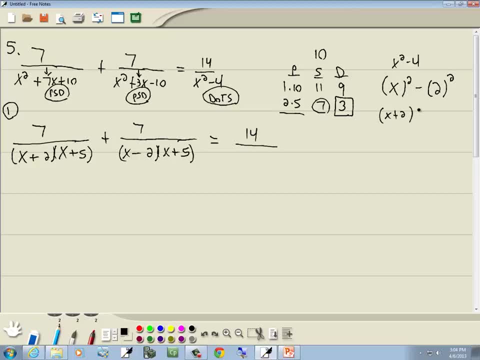 Now we take what's inside our first set of parentheses, we add what's in our last and we take what's inside our first and we subtract what's in our last. I swear there's more noise where I live: Trains, sirens. 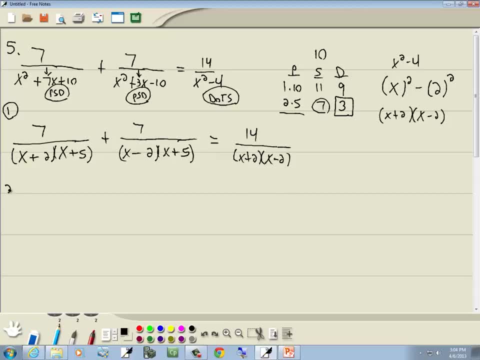 Okay, step two: Figure out your LCM and then multiply everything by it. We'll start with our first factor, the X plus 2.. I'm looking for the greatest number of X plus 2s in a single denominator. There's one here, none here, one here. so greatest number of X plus 2s is one. 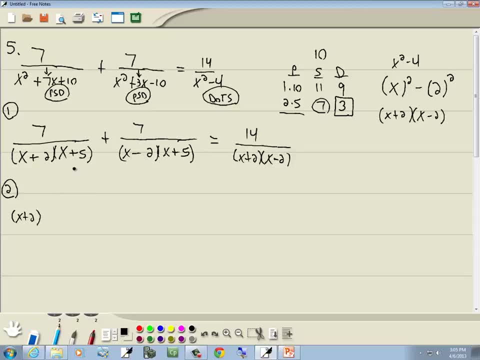 I go to my next factor, the X plus 5, and I'm looking for the greatest number of X plus 5s in a single denominator. There's one here, one here, none here, so greatest number of X plus 5s in a single denominator. 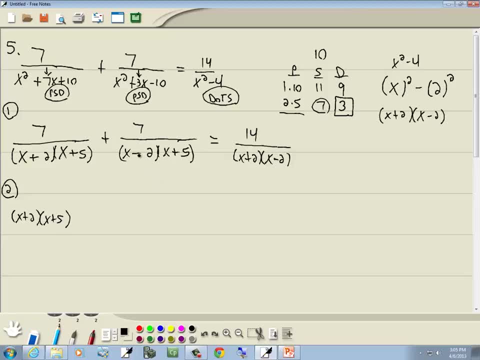 Then I go to my third factor, the X minus 2.. And I'm looking for the greatest number of X minus 2s in a single denominator. There's none here, one here, one here, so there'll be one. So that's our LCM. 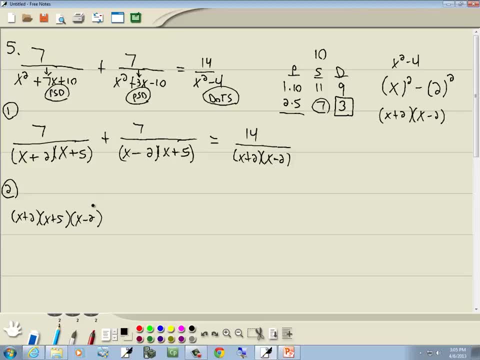 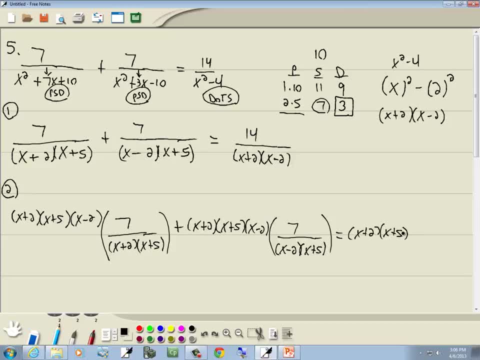 And then we'll multiply it times our fraction on the right side. Okay, let's see what cancels. This x plus 2 cancels that x plus 2.. This x plus 5 cancels that x plus 5.. Over here, this x minus 2 cancels that x minus 2.. 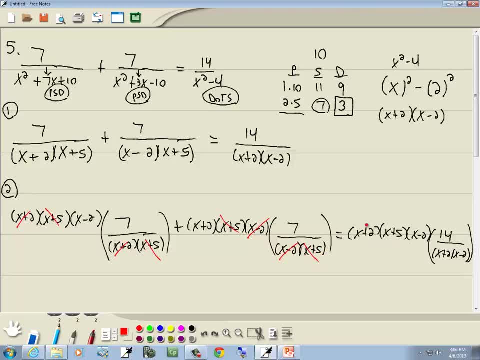 And this x plus 5 cancels that x plus 5.. And this x plus 5 cancels that x plus 5.. And this x plus 5 cancels that x plus 5.. And over here, this x plus 2 cancels that x plus 2..